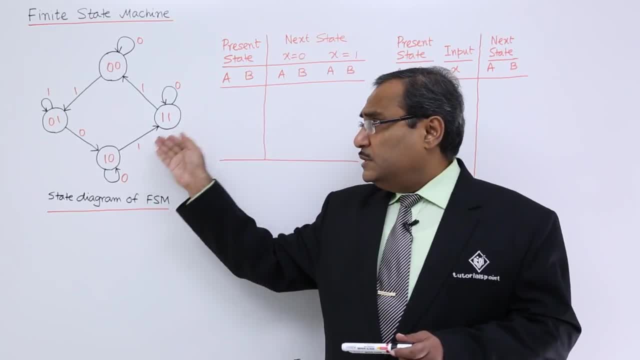 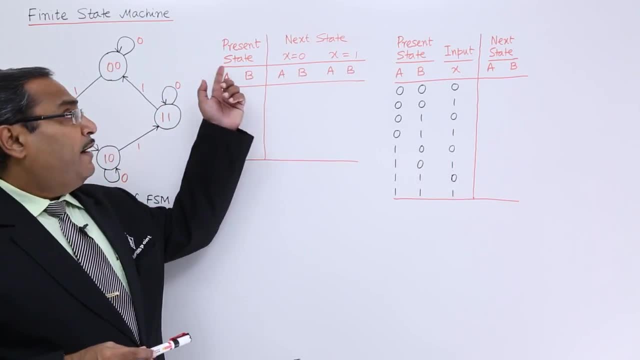 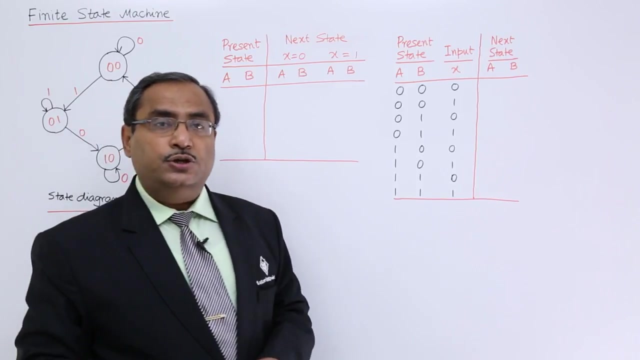 diagram of one FSM. So this state diagram can also be represented in a table. So here you can find that here we are having the headings like finite state, which is being represented by A and B, and then next state, for x is equal to 0 and for x is equal to 1.. So this table is incomplete. 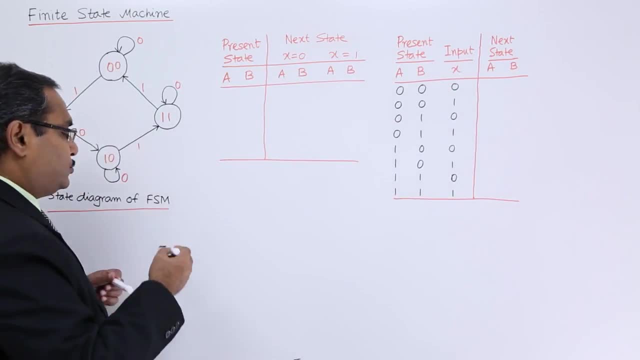 So let us complete it at first. So we are writing this one. all the present states will be 00,, 01,, 19 and 20.. So we have written all these dramas. So, on the electronic change, this is being represented. 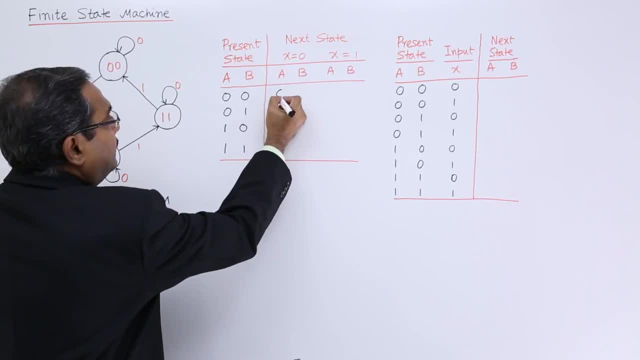 as uniform. So the input signboard is 0, and the top is 1,. this is a shift of était with isஆ: 0,, 1,, 1 and that is the availableabel performance gedacht bit max values. 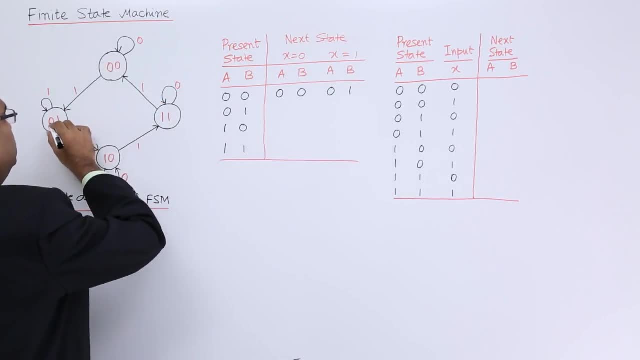 for the block Ω 0 and 1001.. Now I shall go for input 0 and input 1.. Für 00.. für. In this way we have completed the construction of the table. Now this particular table can. 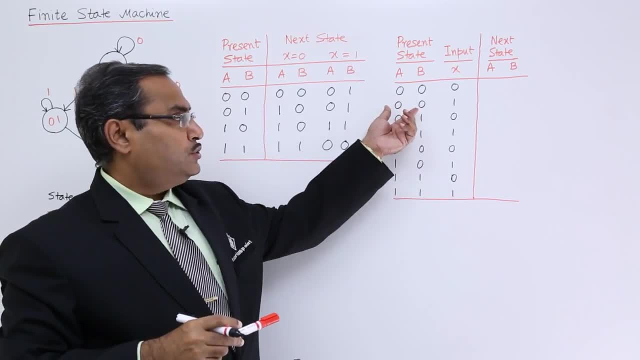 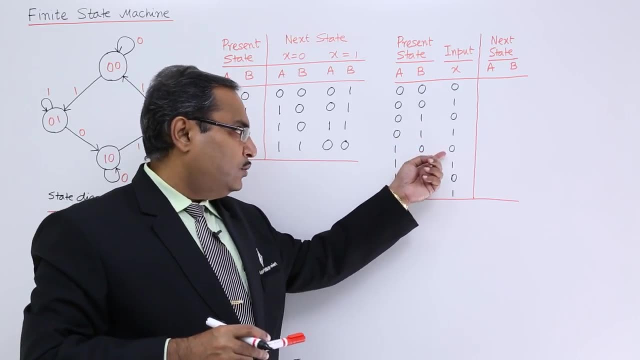 also be represented in this way. So for 0: 0 states, we are having the input 0 and 1.. For 0: 1 state, we are having the inputs like 0 and 1.. For 1: 0, 2 inputs For 1: 1, 0 input. 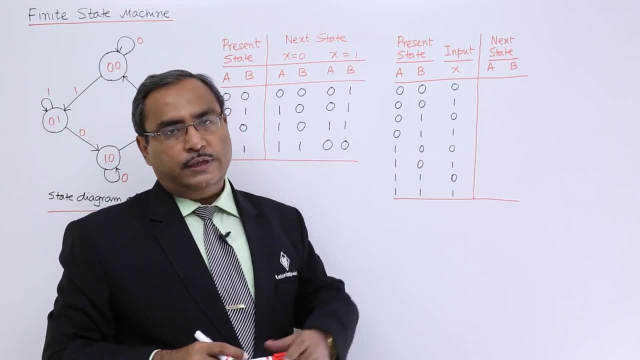 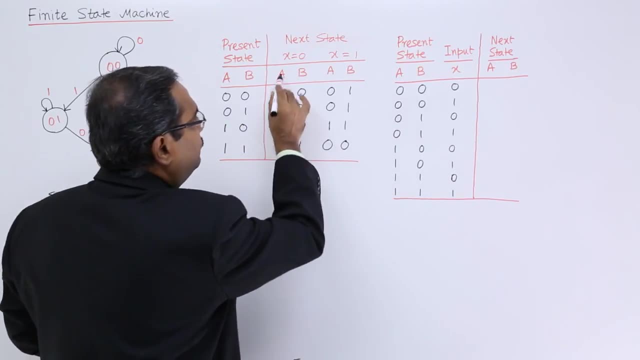 and 1 input. So this table can also be mapped onto this respective table in another form. So let us map that one here. So for 0: 0, for 0 input. we are having 0, 0.. So for 0. 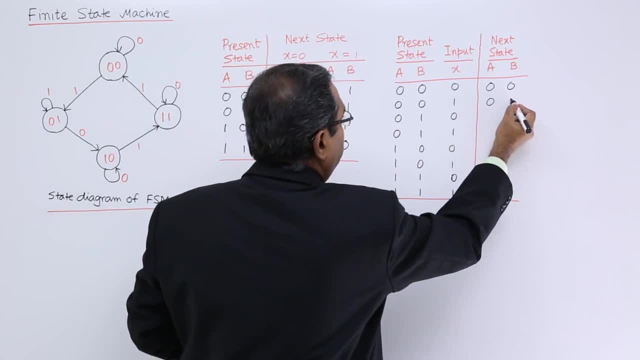 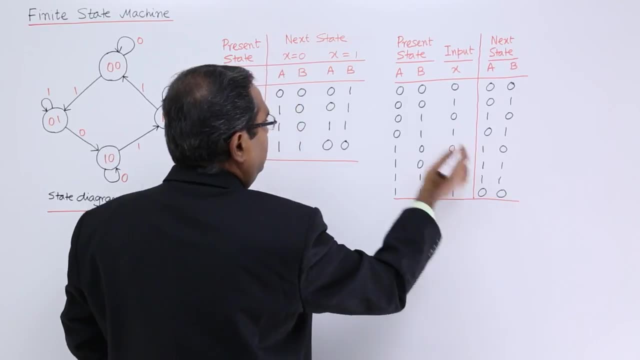 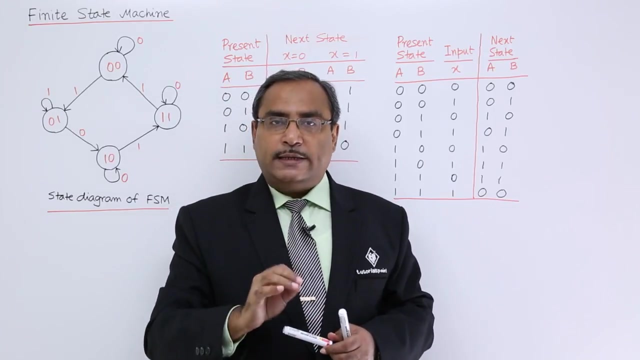 0, for 1 input. next it will be 0, 1.. In this way we can proceed for the rest. Thus, this table has got mapped onto this respective table. So in this video we have discussed that. what is a finite state machine? 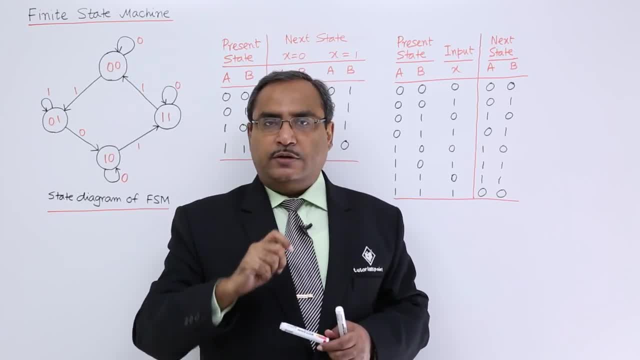 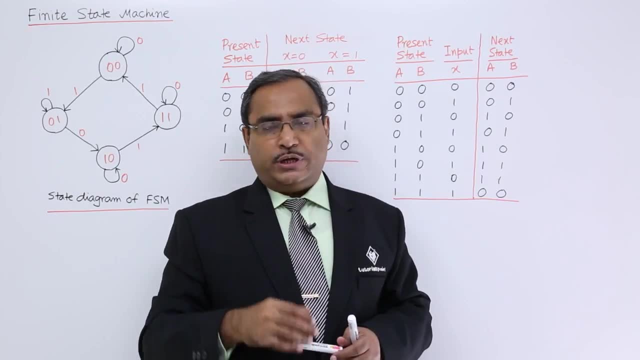 How can we map it, How to represent that one in the form of state transition diagram And how to represent that one in the form of tabular representation? In the next video, we shall implement this FSM using FIPLOPS. Thanks for watching this video.